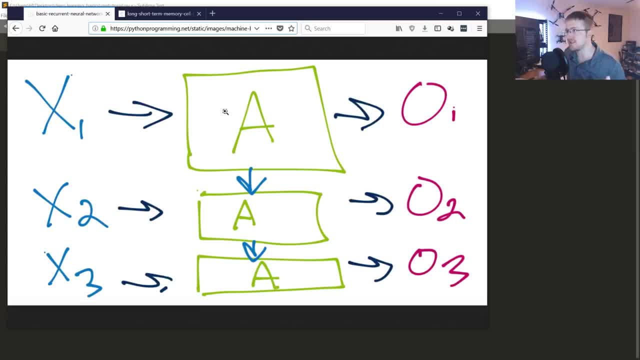 sequential data is passed in, let's say to one of these cells, And then the cell does two outputs to two locations. It outputs one to the next layer but two, And the next layer could be the next. you know, it could be input to the next recurrent type of layer. 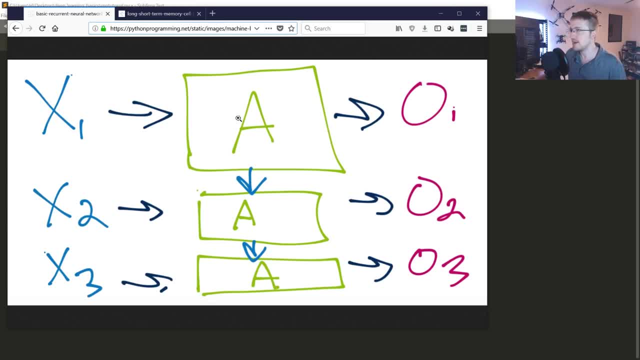 Or it could be the output layer or a dense layer, Who knows? But anyways, each cell is going to output somewhere to another layer, but also down to the next node in the specific recurrent layer. Now where are these output to? It doesn't necessarily have to be to the next thing down, And then it. 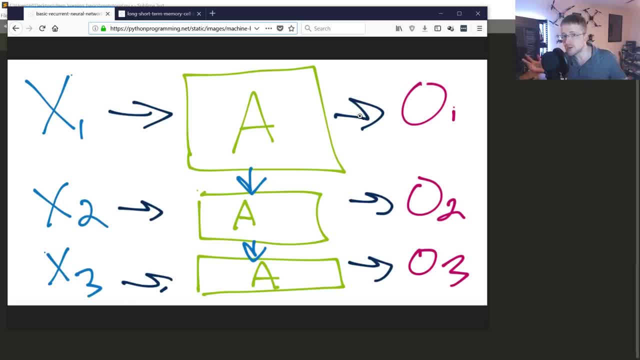 also doesn't have to only go in one direction. You could have bidirectional recurrent layer, For example, and you can get really crazy with the, with the order of things and where data gets passed and stuff, But in general this is a super basic one. So a another way to look at it is like this: 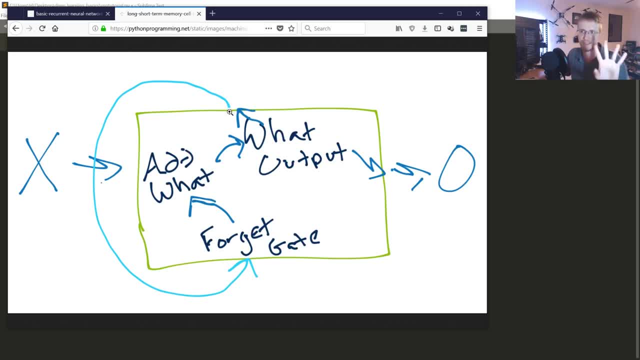 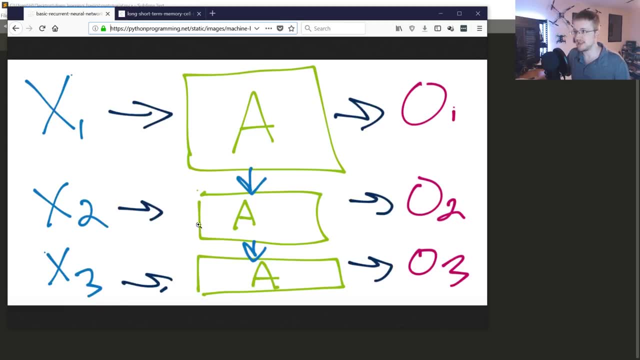 is one cell And so so let's say you've got. basically. let's say this is like the second one in the layer. So let's say it's like we're looking at this cell right here. So this green box is this cell here. OK, So basically some, some data has come from the previous cell. It's wrapped around. 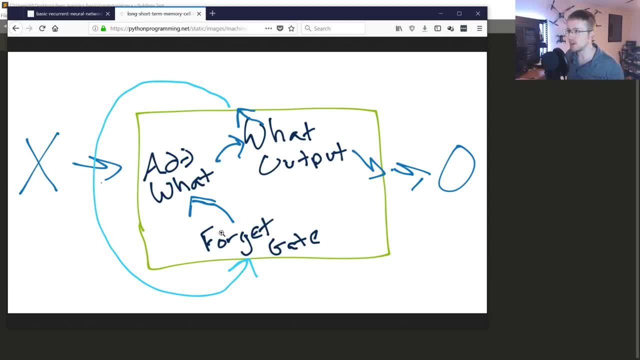 here. It's coming in, And the LSTM cell that we're looking at here. it chooses: OK, What do we want to forget from the previous node? Then there's input data coming in. OK, Based on this input data, what do we want to? 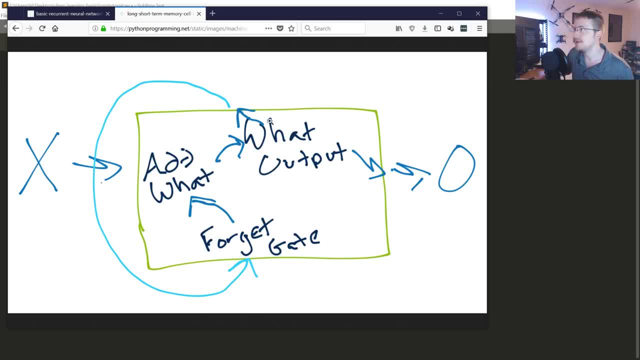 add to this bundle of info that we've got, And then finally, OK, What? based on this bundle of info, what do we want to output to, both the next layer and the next node that we want to output to? So that's the task of the LSTM cell. 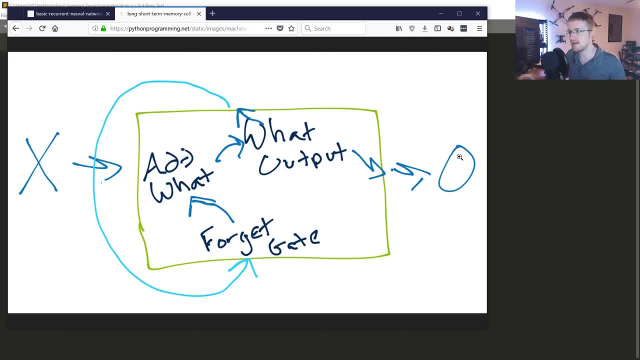 Now, obviously This is the LSTM cell. Now, obviously This is the LSTM cell. Now, obviously That's pretty complicated, especially when you know all these things, like the whole point is to eventually just pass along like a scalar value. So how do we do that? Very challenging stuff. 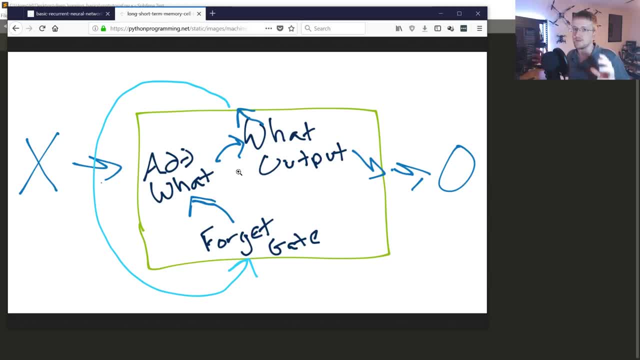 If you want to learn more about how LSTM cells work specifically, there is a great timeless write up on the LSTM cell. I link to it in the text based version of the tutorial, So definitely go check that out if you want to. Otherwise, let's get into writing our own basic recurrent. 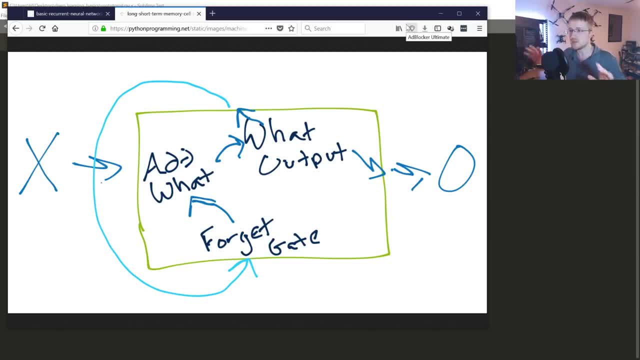 neural networks. So what we're going to do in this video is just do a really simple one, just so we can get the idea of like what really how easy a recurrent neural network itself is. But the really the hard part with recurrent neural networks is getting your data set structured in such a way. 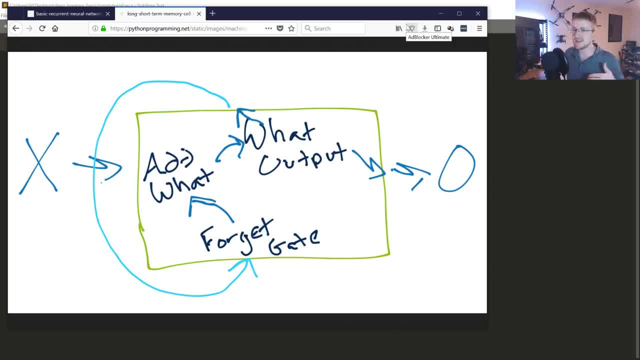 because the type of data that you're going to be using typically doesn't have targets. It has, it's just time series, It's just informal kind of data and we don't really have, you know, what are we actually trying to point this to. So there's usually 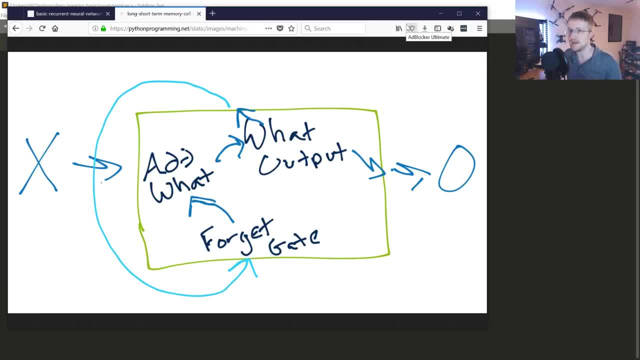 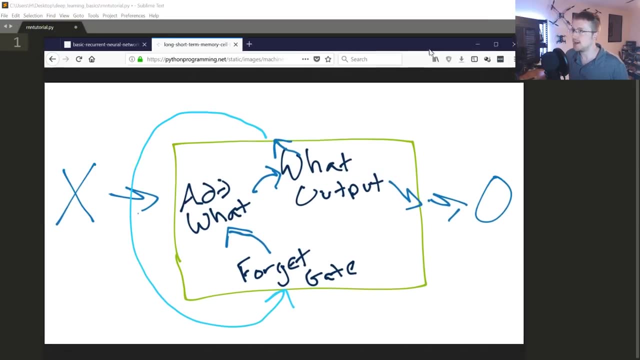 A huge amount of pre-processing involved in when you work with recurrent neural networks. So what we're going to do here is just use a simple MNIST example and in the next tutorial we'll do a realistic example with some time series data, specifically with cryptocurrency prices. So yeah, 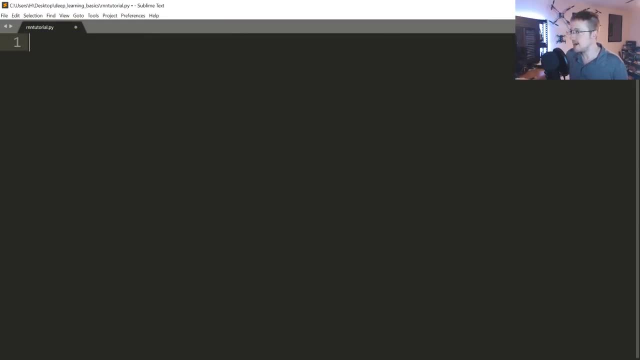 Anyway, I'm going to minimize this and let's begin with some imports. So import tensor flow. as t jerk always does this to me: Tensor flow is tf, fix that. Then we're going to go from tensor tensor flow dot, keras dot models, We're going to import the sequential type of model from tensor flow dot keras dot layers. We're going. 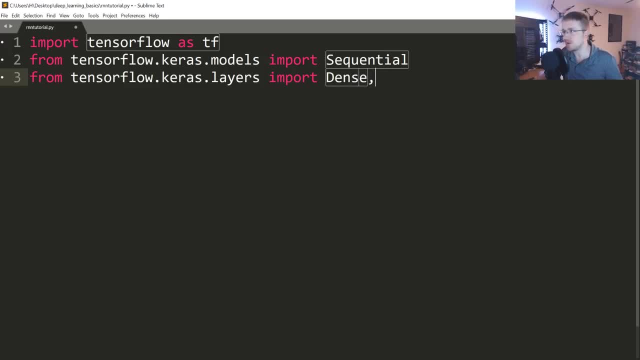 to import the dense layer one, because the output layer itself needs to be a dense layer, But also we are going to end with another, like a realistic, you know, a dense layer before the output layer. That's a pretty common operation to do. Then we're going to have some drop out, just so nothing gets overly weighted, and the LSTM. 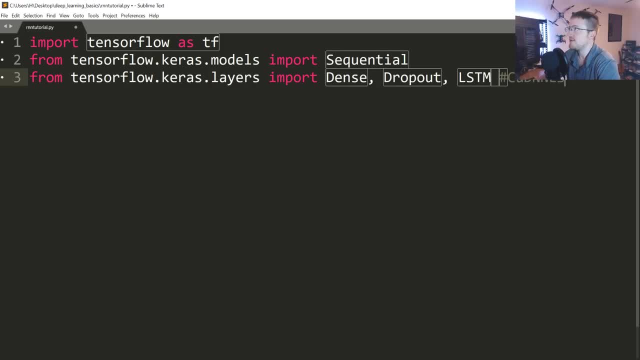 cell. I am going to comment here. If you are on the GPU version of tensor flow, check out the QDNN LSTM cell. So, even if you are on the GPU version of tensor flow, this LSTM cell will indeed run on your GPU, But the QDNN LSTM cell is even more optimized and it's like five plus times faster. 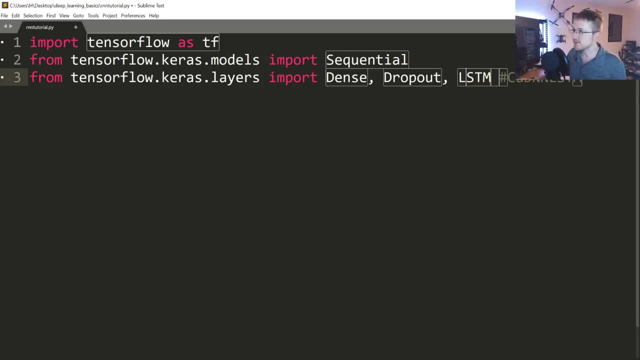 Even though both run on your GPU. If you're on the CPU version of tensor flow, well then you know you're going to this tutorial like this model is going to take like five hours to train or something either way, Okay so. so those are the things that we need, and now we need the data set. So we're 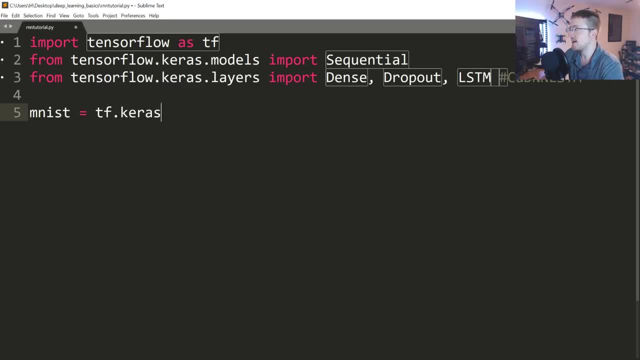 just going to grab mnist real quick. So mnist is equal to tf, dot, keras, dot, data sets, dot, mnist, And then we just need to unpack it, So it's just to these two tuples, and then it's x train, y train, then it's x test, y test, And that's mnist, dot load underscore data. So again, my apologies. 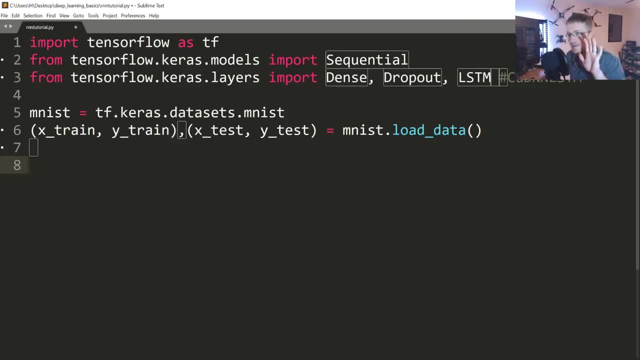 for using mnist. but I think it's better to do it: make this one as basic as possible and then in the next one we'll get in, Because honestly, it would take us. it's probably like the next one's probably going to take us two, three, maybe even four parts just to get to. okay, now feed it through the neural. network, And that's the easiest way to do it. So just remember, mnist is equal to tf, dot, keras, dot. tf, dot, keras, dot mnist. And then you just need to unpack it. So if you're on the GPU version of tensor flow, well then you're going to need to unpack it. So it's just to these two tuples and then you're going to. 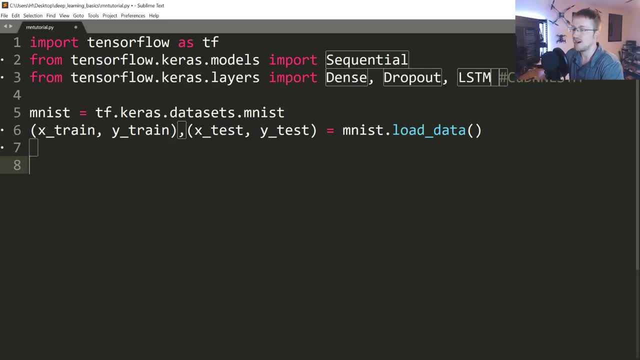 need to unpack it. So it's just to these two tuples and then you're going to need to unpack it. So it's just part. really feeding it through is is not too hard, so, uh. so, for example, let's do- uh, let's just do a. 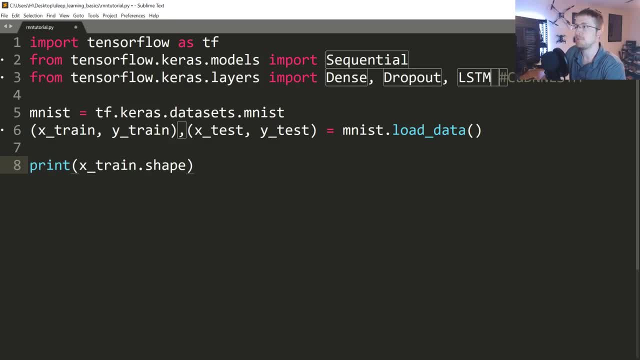 print x train dot shape and then we should be able to do to deduce this uh from uh the above, but x train, and let's just get the first sample dot shape, just so we get idea what we're dealing with here. so, um, so we can see, we've got 60 000 examples of 28 by 28 images. 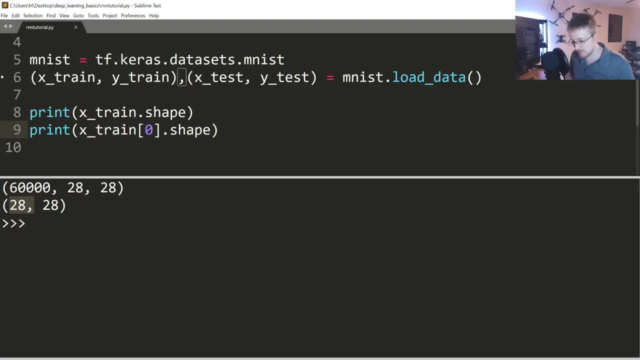 and, of course, the zeroth element is just 28 by 28.. so take a minute pause and think about: okay, so this is our training data and it's already in sequences for us, right? and what are the sequences? well, it's in sequences like: what is this? 28 by 28? well, it's 28 rows of 28 pixels per row. 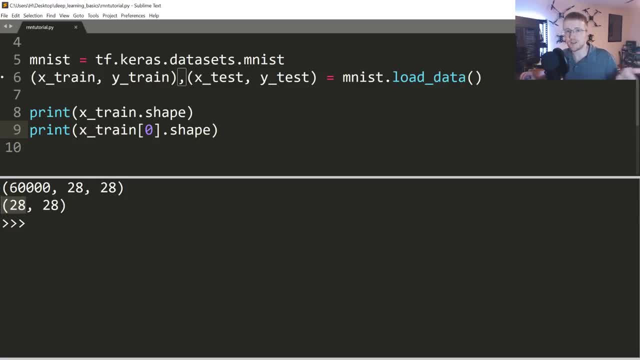 so we could in theory say each, each row is a part of a sequence, and if you were to take the first row and then take the second row, and then take the third row, and then take the third row row, and then kind of scan downwards, could you figure out what the number is? probably, um, so the 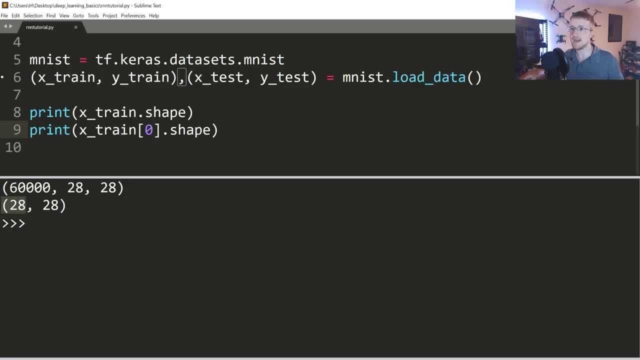 so the hope is that a recurrent neural network could actually do this and, um, maybe even more so. we should see that it could plausibly do it better than a deep neural network. but we'll see. um, the more important thing is just to show the recurrent net anyways. um, but yeah, so, so that's the sequence. 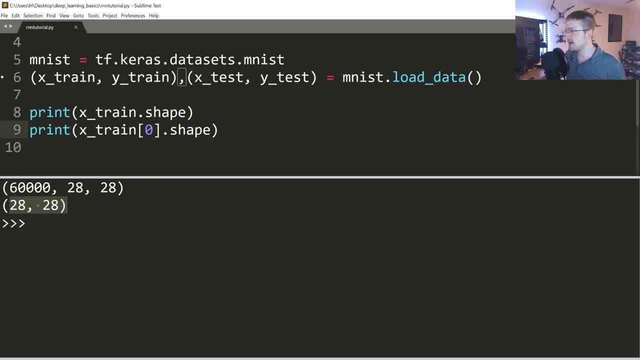 it's a sequence of rows of pixels. um, that we're, that we're going to be feeding through this neural network. so now we want to build the actual model itself. so we're going to say: model equals- i'm going to give us some space here- model equals, and it's just going to be that sequential type. 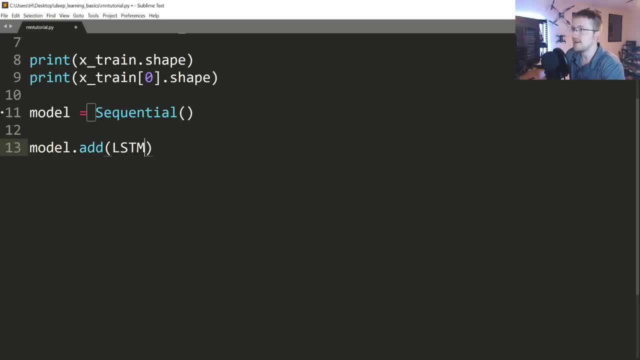 of model. now we're going to do modeladd and we're going to add in an lstm cell. how many uh or lstm layer? right, how many uh cells do we want to have? we're just going to use 128 for now. we're going to specify the. 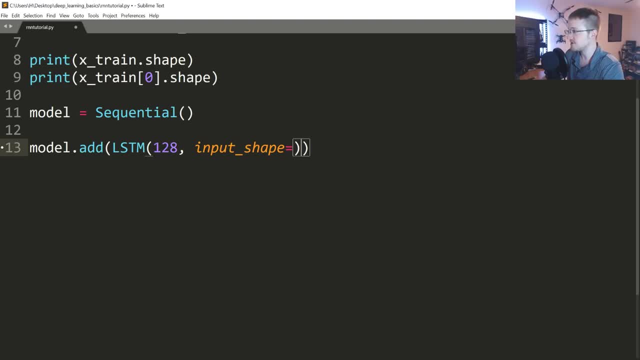 input shape, and that is 28 by 28. we already kind of know that, but we can make this somewhat dynamic by doing x, train, dot, shape, um and then one colon. so then we can pass an activation function and we'll use our good friend rectified linear. 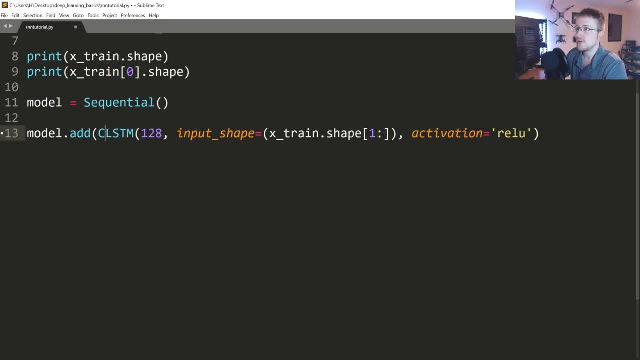 and again: uh, do check out. ku ku dnn lstm. uh, i'm just not going to do that yet. i'll probably change it before we run it because it is really, really fast, but for now we'll just keep it. oops, didn't mean to move that, we'll just keep it here. 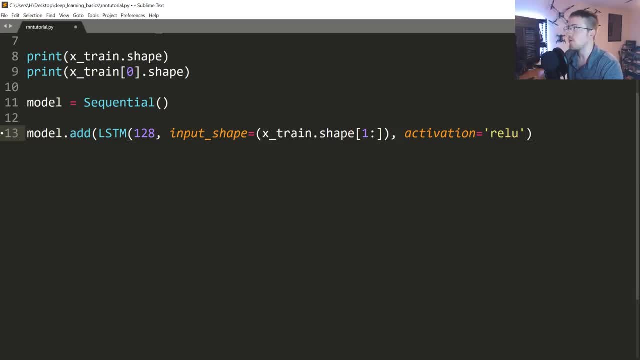 okay, so the next thing that we want to do is one more parameter, which is return underscore sequences, and that's going to be true. so do we want this layer to return sequences like it was input, like sequences were input, or do we want this layer to return something flat? 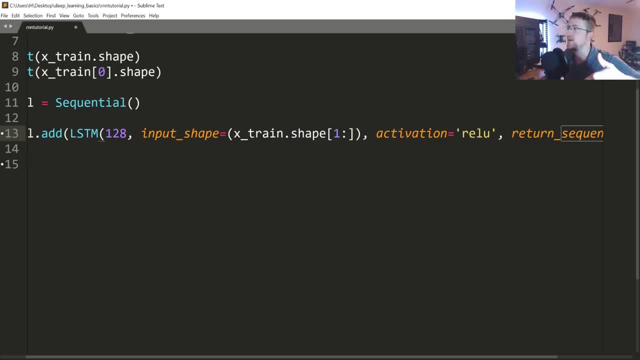 right. so if we're going to a dense layer, we wouldn't want to return sequences, because a dense layer is not going to understand what the heck's going on. but if we're going to another recurrent layer, we definitely want to return those sequences. this is just a long line. 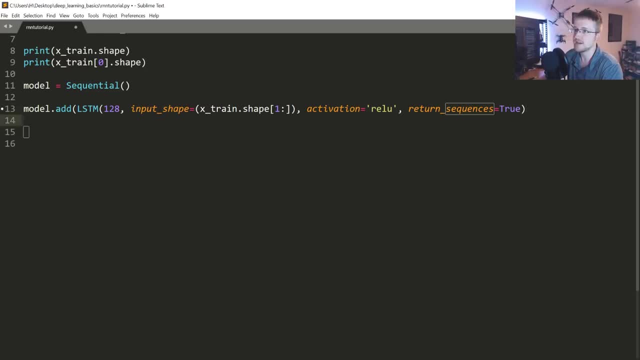 anyway, okay. so so that's one of our uh layers, and then we're just going to do model, that ad, and we'll throw in a dropout, because that's what you do. so we'll do a 20 drop out there and then we'll do another layer. so, modeladd, we'll add an lstm layer, we'll do another 128. 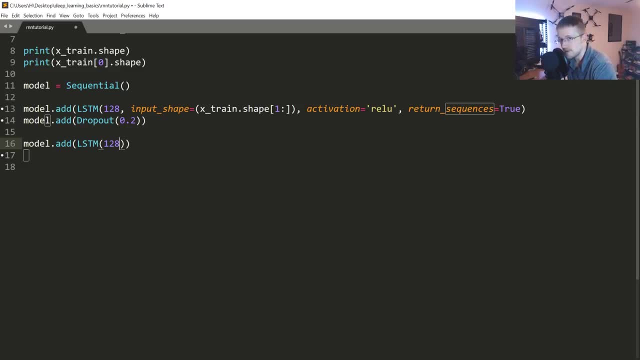 we don't need to specify input shape. in fact i don't know why we ever had to- and then we will pass an activation function here. activation equals rectified linear. we'll do a dropout. i'm just going to copy and paste, copy paste. and then let's do a modeladd. 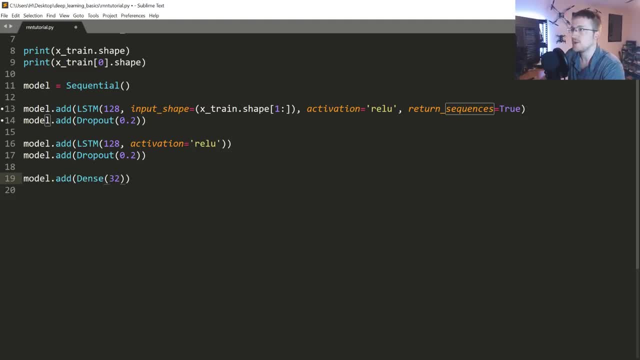 we'll add a dense layer, we'll make it 32 nodes, uh, and then activation- gosh, can you guys think of what activation? oh yes, that's right, rectified linear, uh. and then we'll do a dropout, and then we'll do, we'll go to the final dense. 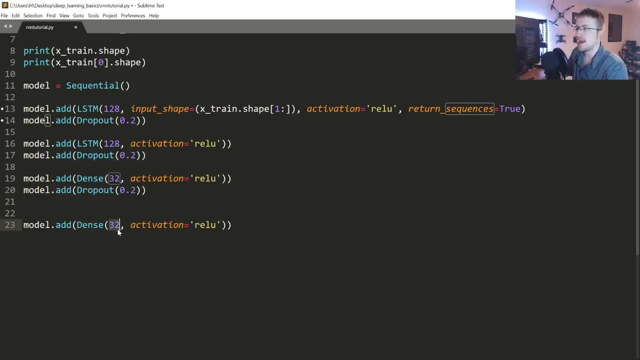 layer. so i'm just going to copy this, paste and i'm just going to hard code in 10.. it's just how many classes do you have? so we're just going to go with 10.. uh, the activation should to be rectified linear. it should be soft max at this point. and okay, i think we're done there with. 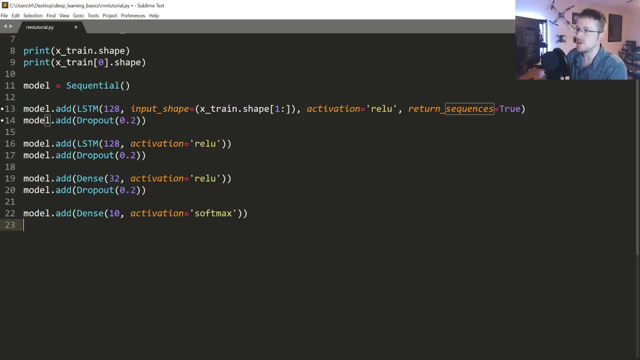 like, at least with our, you know, model structure. now all we need to do is do the compile and then the fitment. so, to do the compile, we're going to have an optimizer compile, compile anyways, uh, tf, dot, caros, dot, optimizers, optimizers, dot atom, and we'll just specify a learning rate of one e. 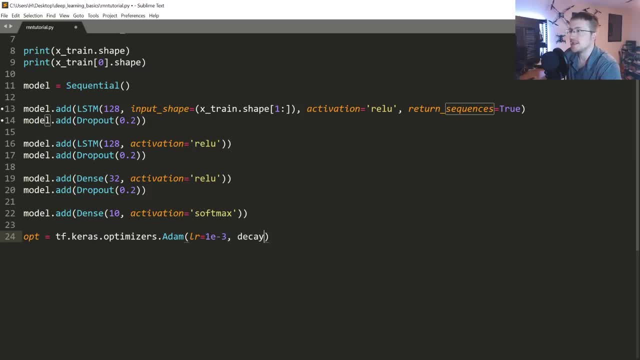 negative three and then we'll do a decay. well, we haven't really talked about decay, but we'll do a decay. uh, one e negative six or something. uh, probably that's too small. maybe one e negative five, so a decay is just over time. uh, we'd probably, like you, want to start with a larger learning rate. 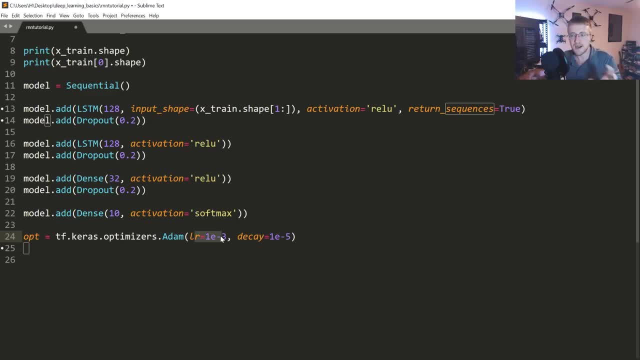 to take those large steps that you want to take and then, but over time, uh, you'll kind of find this like local spot, but probably you're. if you took smaller steps you could do even better. so if you keep taking those big steps, you're going to keep bouncing around that little. 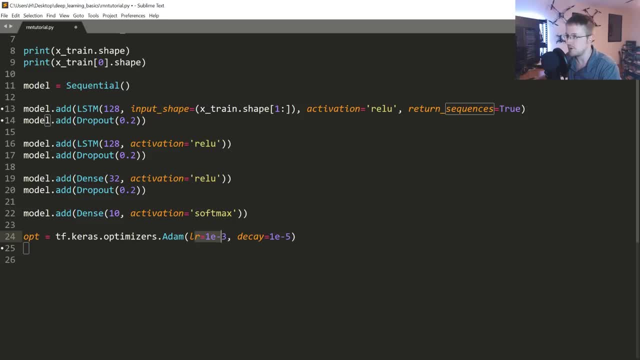 u shape, but if you take a smaller step you could plausibly do better. so, anyways, that's what decay is about. it's just over time, every batch it's going to decay the learning rate a little bit, so it's going to keep shrinking that learning rate, and so you'll take smaller steps anyways. 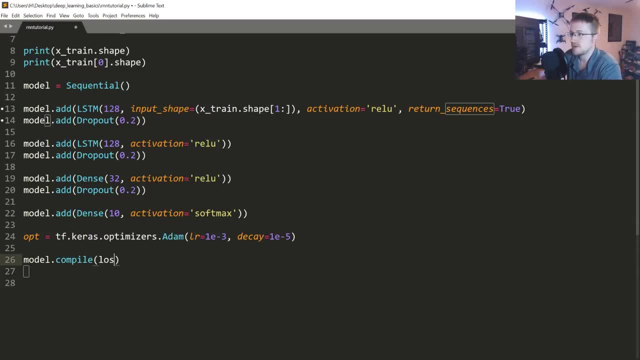 model dot compile and we'll say: loss equals sparse, categorical cross entropy. i just want to say, uh, they did add a shorthand for mean squared error. squared error use. you know, that's one way you can measure loss, and they said it was. it's now you could use mse. 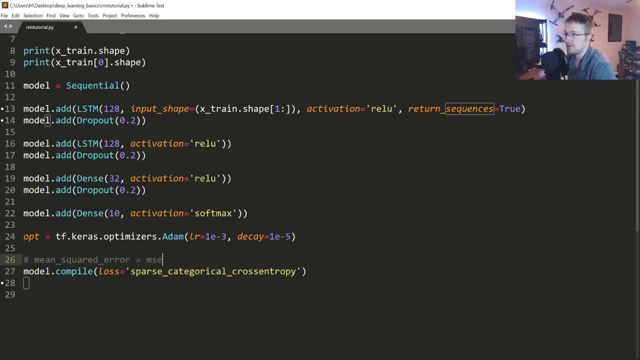 um, i'd really like it if they added shorthand for all of them. someone tell me below if, if they have- and i just don't know about it, but you know- i'd like to be able to say scc. that'd be nice. i hate typing that out. okay, so we got our loss. uh, the optimizer equals. 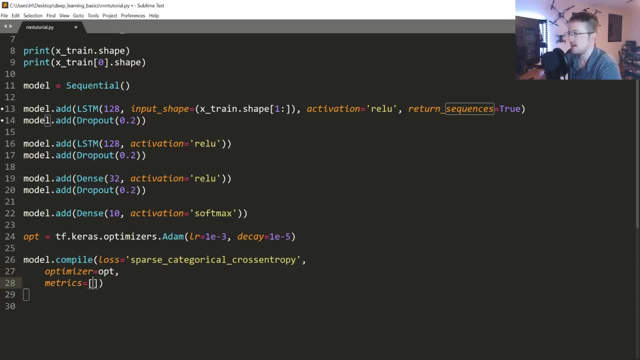 really simple there. and then the metrics that we're going to track here. uh, we'll just go with accuracy. and then finally model dot fit: x train, y train, epochs- we'll do three epochs validation data so we can see it over time will be x test, y test. 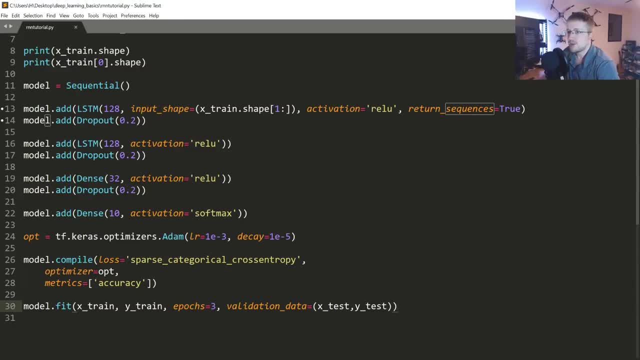 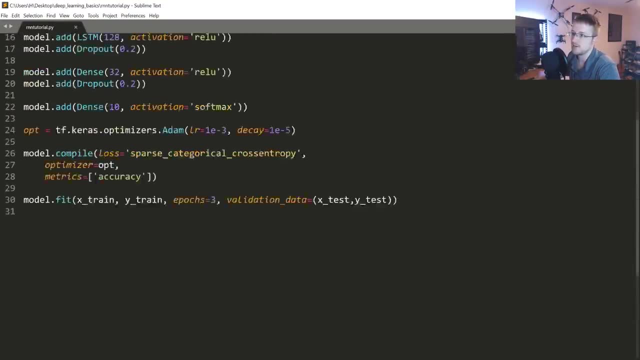 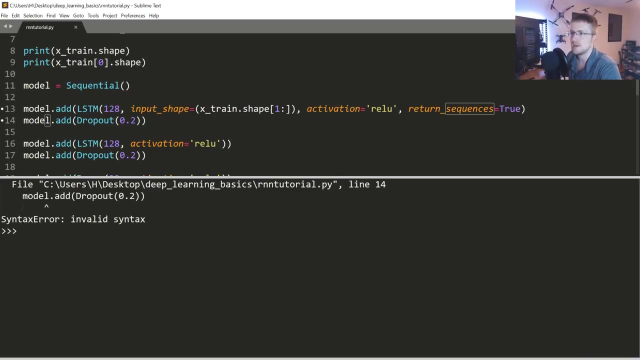 okay, so that should be good to go. hopefully i can run this and not crash the computer, because i know um sublime likes to really get me. so, uh, we'll go ahead and run that. now i'll probably just go through maybe one epoch up, let's see invalid. 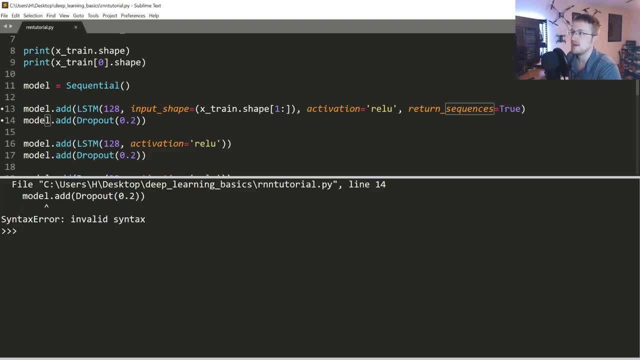 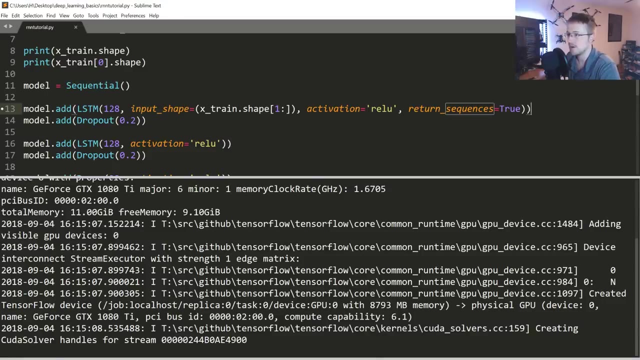 syntax at the dropout. what did we, and maybe not? what line is that 14? did we not fully close this off? we didn't try again with root. okay, things are looking good. so far, all right, and we are off. we are learning. the accuracy does not look very good. 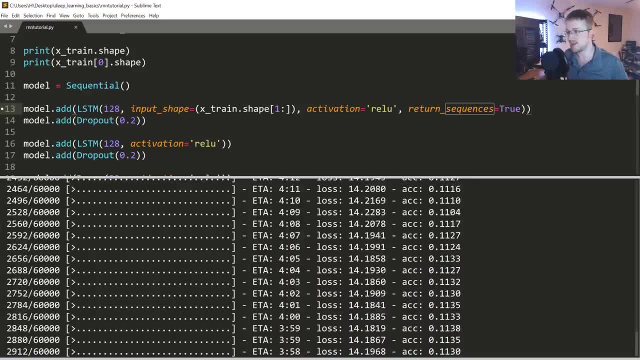 but you can see how slow this is like. this is extremely slow. i would expect accuracy to be a little better even by now. i wonder why this is going so painfully slow. i wonder if i've made a mistake, even because i don't even see loss going down. it almost looks. 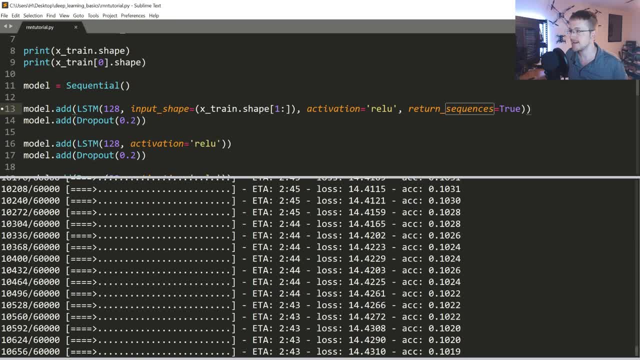 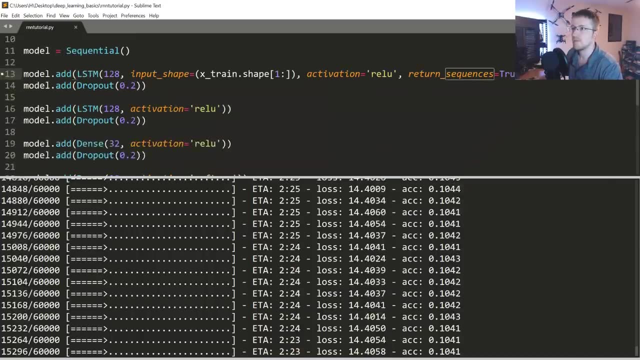 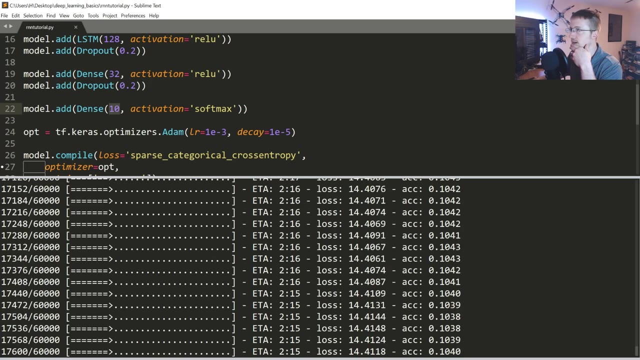 like loss is going up 14.5. i don't know if i've made a mistake, even because i don't even see loss. 14.3938, hmm, no, first i saw this i was like, oh, that's our problem. no, uh, we've got our final dense layer. 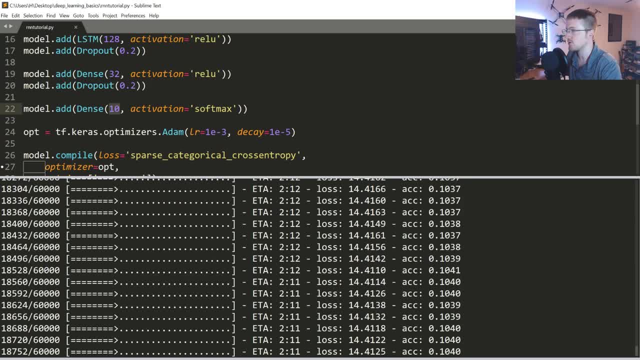 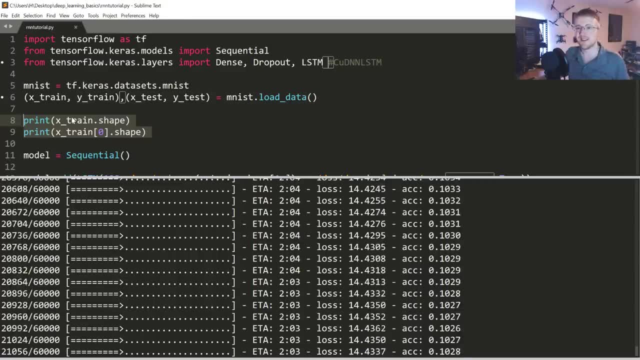 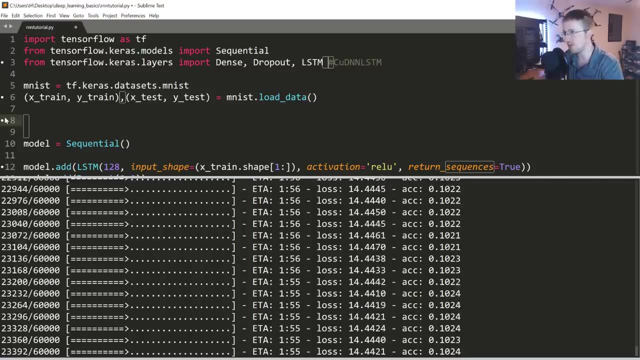 activation is soft max. what did we screw up? we have to have screwed up something. it should be learning much more by now. good, thats good. ok, um, so this is in it. oh, i think i just had a present. I've never done this before, so this is in it. oh, I don't know if we've ever- I don't know that we've ever- shown this, um, but I 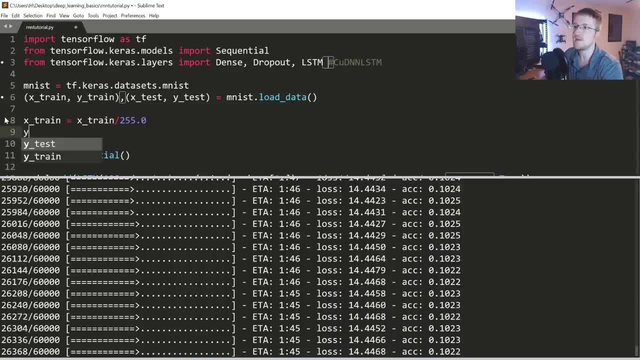 brought it up at least. what aren't we doing here? we are not normalizing this data, so we could use the carre's normalization. or we can just say: X train equals X train divided by 255. XTEST heribles: x, Committee: 255, 255. 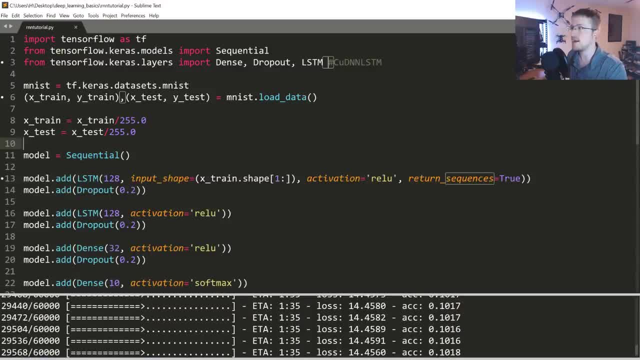 i'm going to save that. the other thing about this process is it's going to bite us full hard be on a board. I've got like 40 degree春 but, like i said, what's the current thing i'm going to do while i have you guys is show you kudian nlstm. so let's go ahead and import. 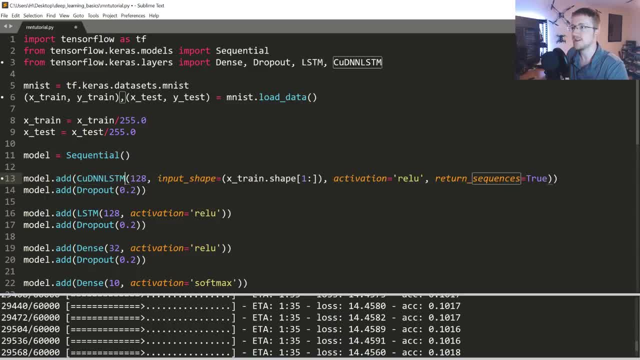 that as well. i'm going to change this to kudian nlstm in this one, and then you, you can't. the kudian nlstm uses a tan h activation function, which is- you can google it if you want to see like the shape of it, but you should be able to rectify linear. you should still be able to get. 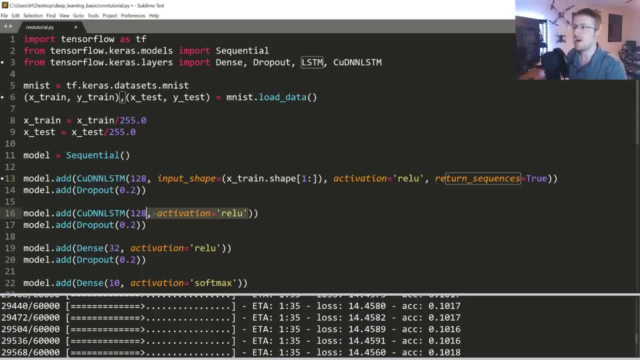 a good accuracy here, but the problem was def. i almost kind of. i almost kind of want to show you guys, because i know some people aren't going to be able to run this if they're on cpu and they just want to learn, so i guess i'll just rerun it. um, but we can even see. so like this: did not train and 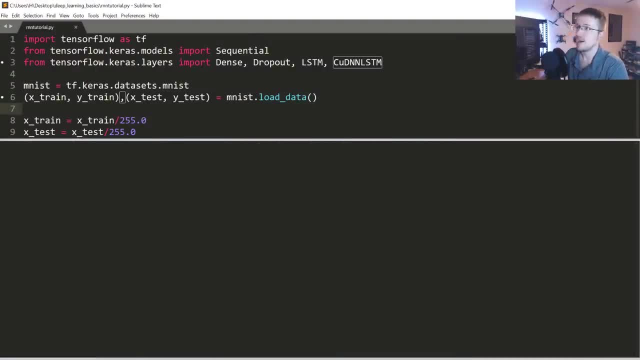 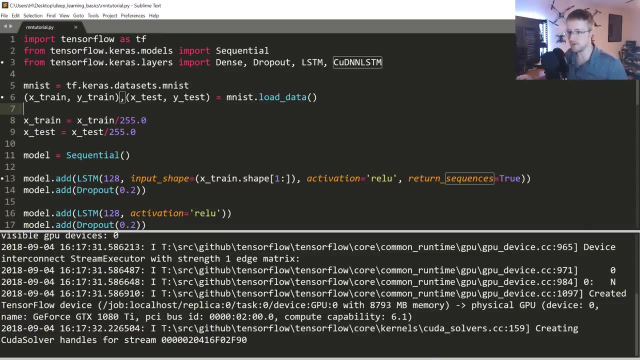 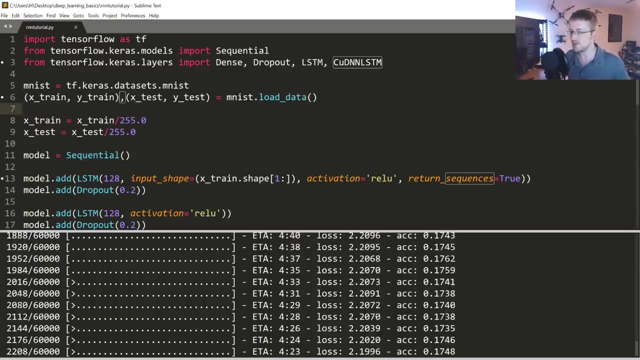 hopefully that was the problem. wouldn't be really sad if that's not the problem. um, but the re, almost certainly the reason this didn't train is because we didn't scale between zero and one. so let's see the example. uh, yeah, i mean look how much faster it's learning now. all we did was scale it between zero and one. 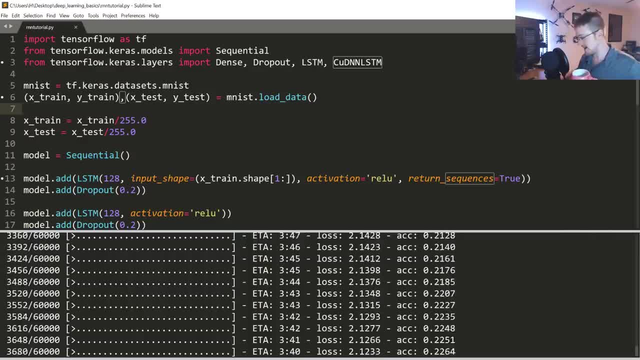 that's how huge of an impact that makes. um, so yeah, it's super important, okay, so i'm going to go ahead and break. well, i guess i don't have to break it, but i'm going to show you guys now, kudian and lstm because it's so fast. anyways, paste, paste, and then i'm going to. 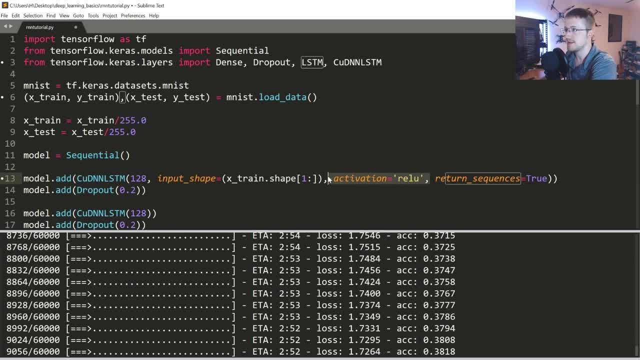 delete this and delete this. whoops, we do want to have that, though. so see, we're already at like 41. i'm sure we're going to get into like the 90s or something, um, but let me eta two, three minutes. so now let's run this one. hopefully i'm not going to crash the gpu. sublime is pretty bad, i probably. 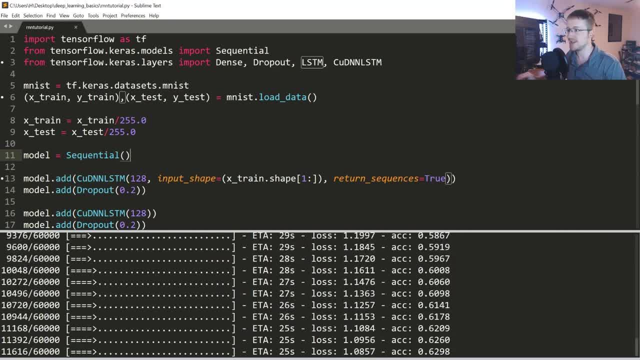 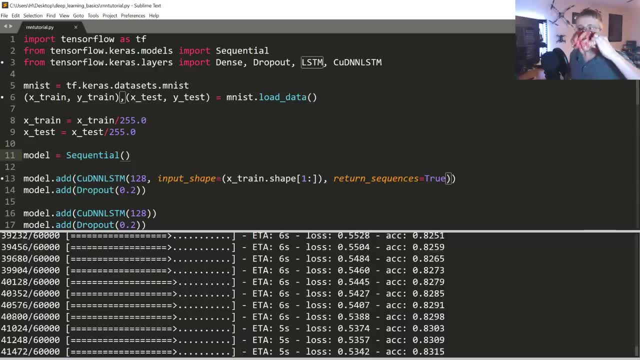 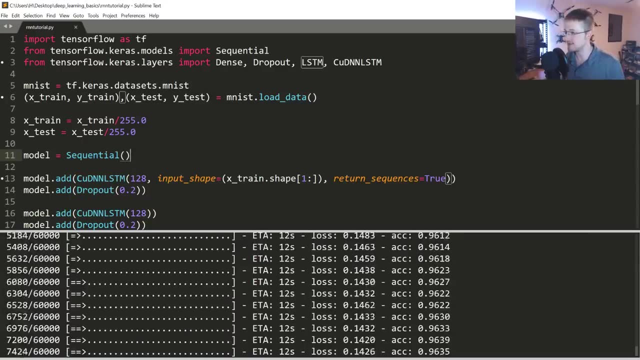 should be running this in a console instead. but whatever, look at this. look how fast. this is the best, the best thing ever. what a great little addition. i mean, recurrent nets are so slow. this kudian nlstm cell is just glorious. so we're already at an accuracy of- uh, you know 96. 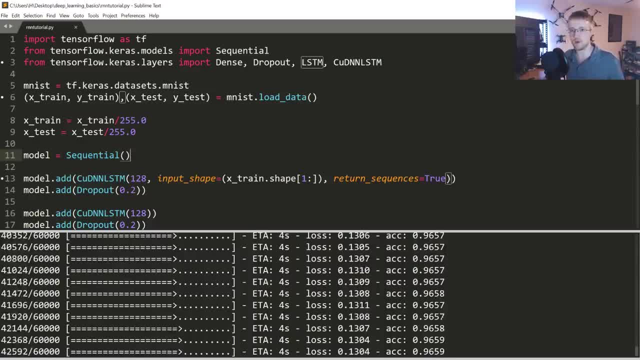 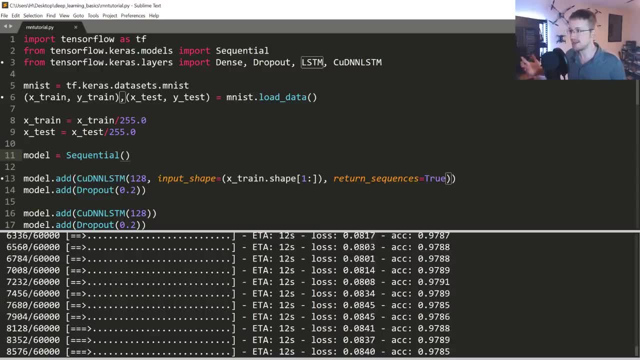 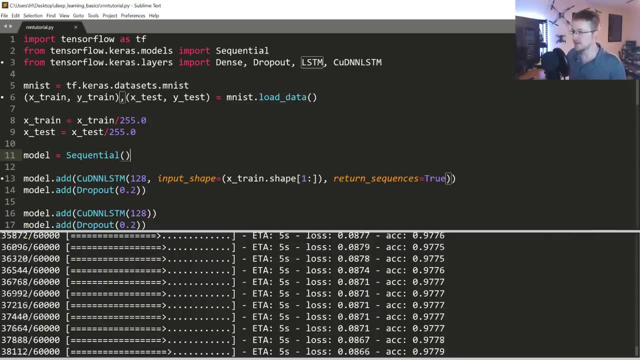 and before epochs were taking i don't know, we were pretty deep into that one and it was like two, two minutes and 30 seconds to go, uh, whereas these entire epochs are taking 13 seconds. that's, that's, that's crazy. um, okay, so i think we're only going to run for three epochs, so i 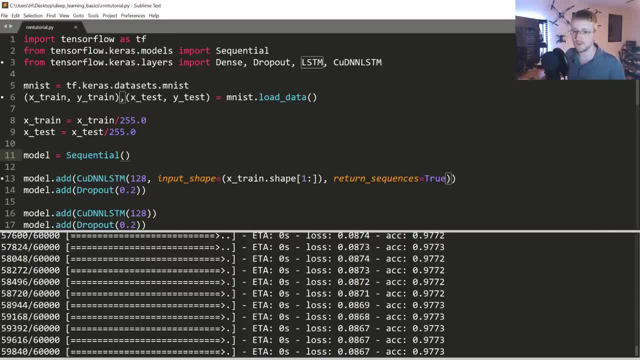 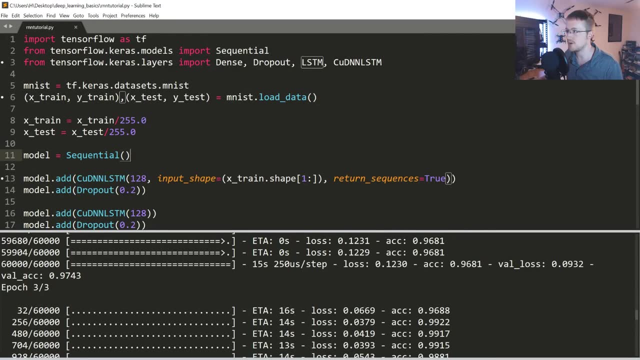 guess i'll just let this one finish. um good, done. so validation. so accuracy here: 97.73. validation actually did better 98.11. um, i don't know if i can get back to the other layers or not. i did want to show like on this. so like on something like this i think the reason why validation. 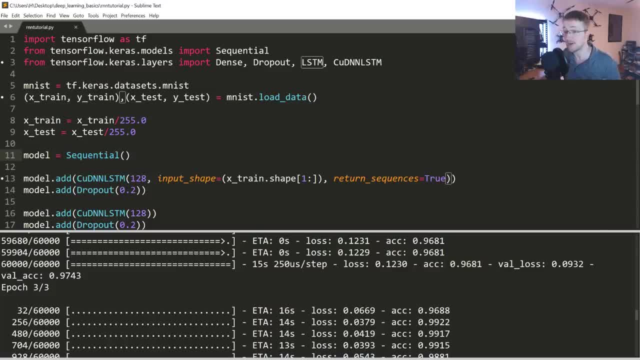 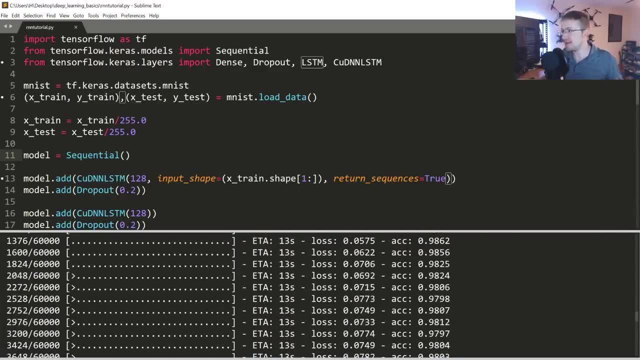 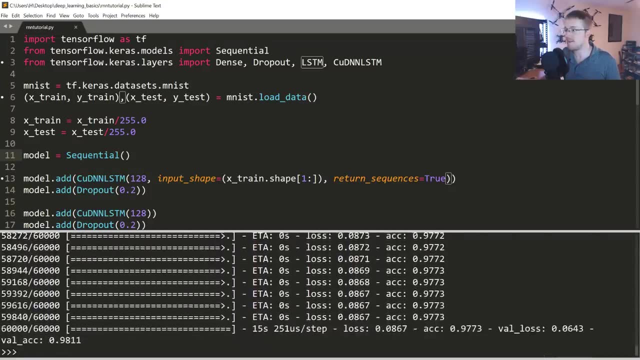 accuracy is higher than accuracy is because this is an average for the entire epoch, whereas this is, like at the end of the epoch. we run it so um, and that's also why, like this is at the, this is an average for the epoch. so then after the next epoch we can see a lot of times our average will. 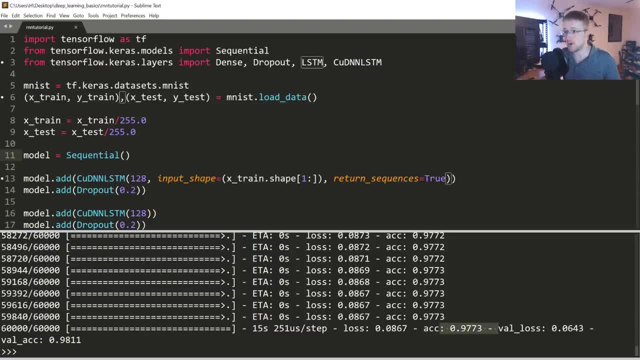 jump quite a bit, um, but even in this case it's still lower than the validation accuracy, which tells me we actually probably could have continued to train because, um, by the end of the epoch we were much, much better. but uh, we could also look at it: in tensorboard is loss still falling and 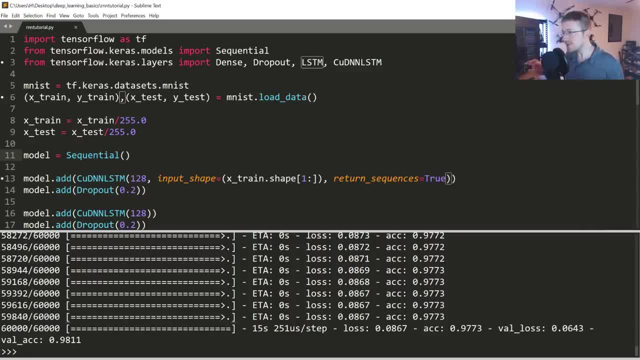 all that. so, anyways, that is all for now. in the next tutorial we will go over a far more complex example of doing this on like a realistic time series data set. uh, because that it just takes so much more work. but i didn't want to bog us down. 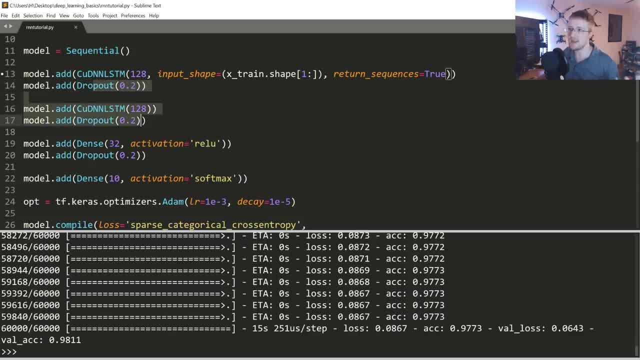 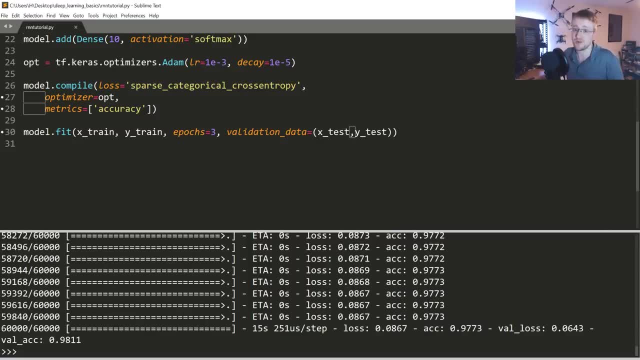 with the pre-processing, uh, without this, because actually you know, feeding it through a recurrent net itself. as long as you have data that's already in sequential form and already has a target, um, it's actually pretty simple, um. so, anyways, that's it for now. a quick shout out to their most. 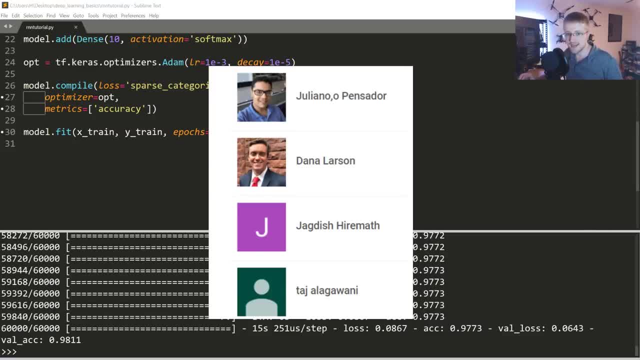 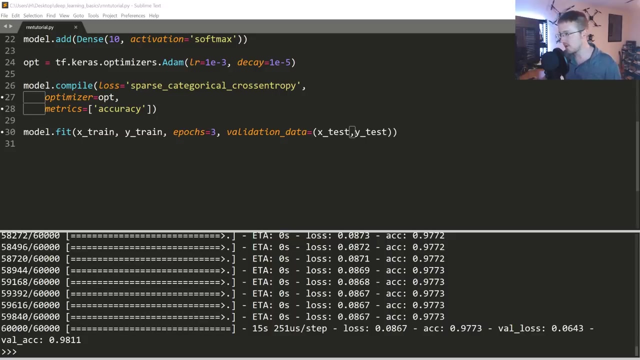 recent channel members: taj jagdish, dana, larry, and i'll see you in the next tutorial. bye, bye. so anyway. that's all for now. if you have questions, comments, concerns whatever, feel free to leave them below. if i did screw something up, in general that is a red flag. i'll see you in the next video. bye, bye. 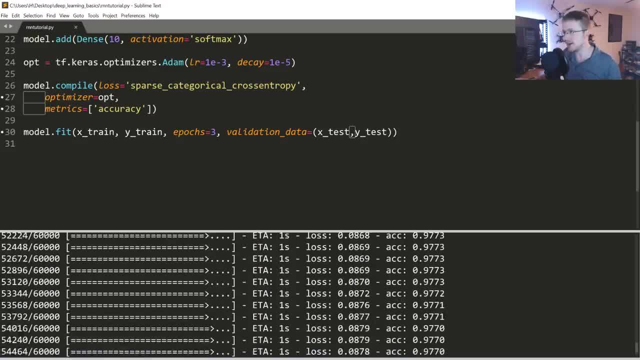 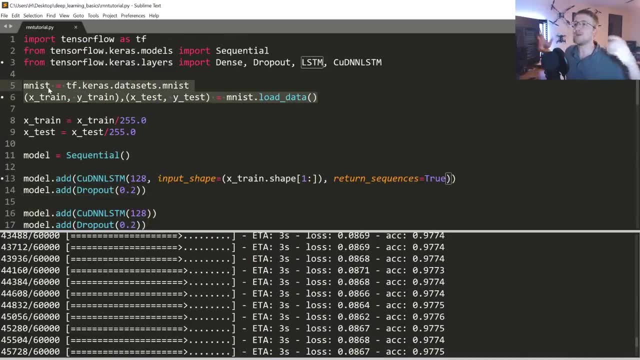 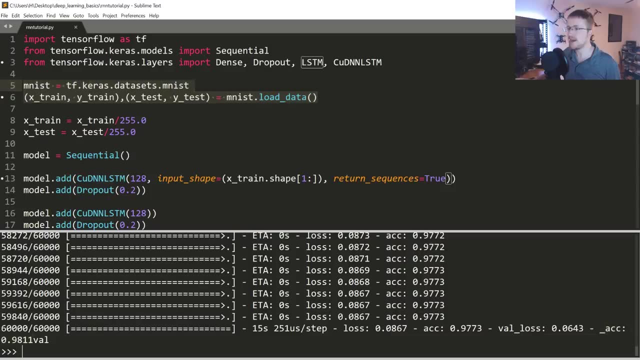 red flag if validation accuracy is higher than accuracy. but i do believe, uh, my explanation before is is why that's the case. also, i'm i'm very confident that their data is prepared correctly. um, but anyways, if that ever does happen to you, that should always be a massive red flag. keep training and make sure that that uh is not the case. 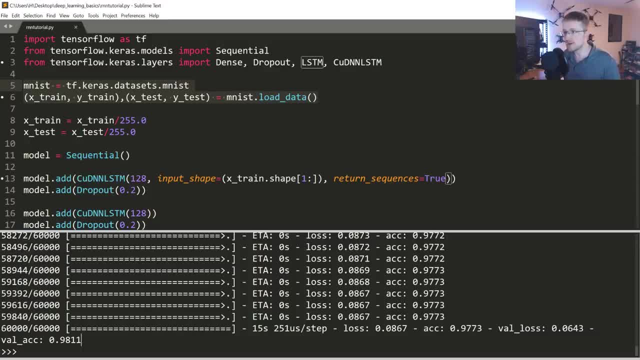 forever anyways. uh, that's it for now. questions, comments, concerns whatever. feel free to leave them below. if you've got any requests for things that you'd like to see in this series, let me know. otherwise i will see you guys in another video.